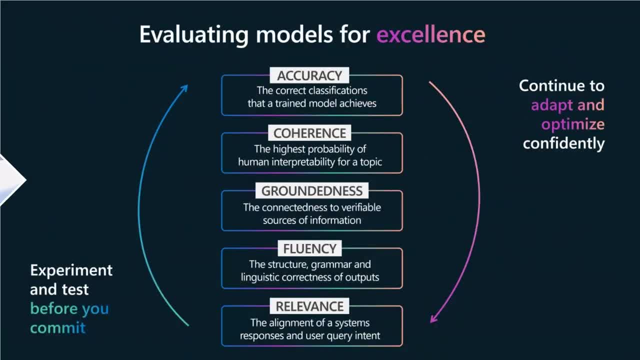 evaluation flows in Azure Studio. Advancements in language models such as OpenAI, GPT-4 and LLM-2 come with challenges related to responsible AI. If not designed carefully, these models can perpetuate biases, misinformation, manipulate content and other harmful outcomes. 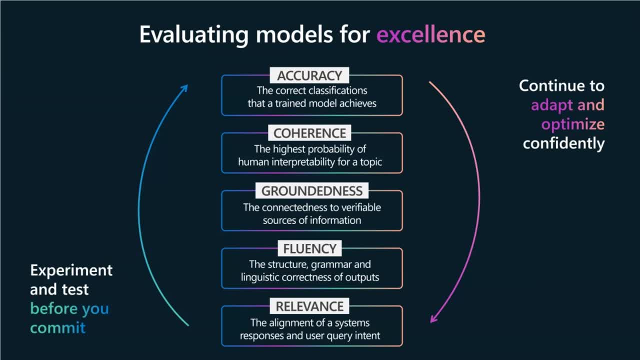 Identifying, measuring and mitigating potential harms associated with these models requires an iterative, multivariate approach. Of course, traditional ML metrics can be helpful when we want to quantify the accuracy of the generated output to the expected output. However, in many cases, 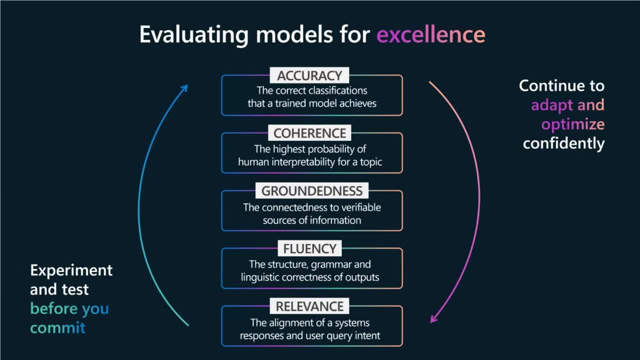 it's important to tackle a variation from multiple angles, using AI-assisted metrics to measure the quality or safety of the answer. Quality refers to attributes such as groundedness, relevance, coherence and fluency of the answer, while safety refers to metrics such as self-harm. 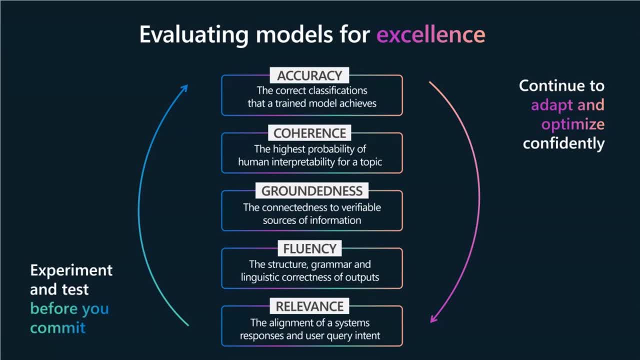 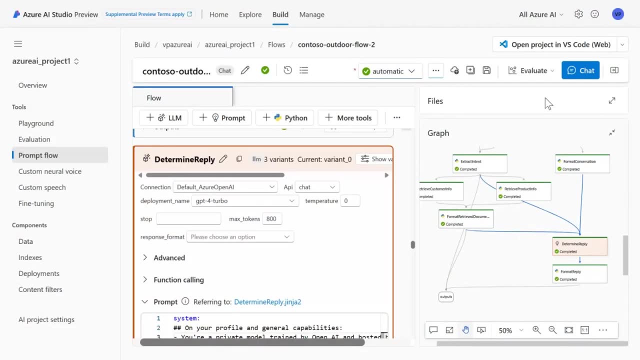 sexual or violence. Azure AI Studio supports several distinct paths for GenAI app developers to evaluate their applications. Ambition you can share using the variation flows in Prompt Flow- Wonderful. Thank you, Takato. As you mentioned being in the field, 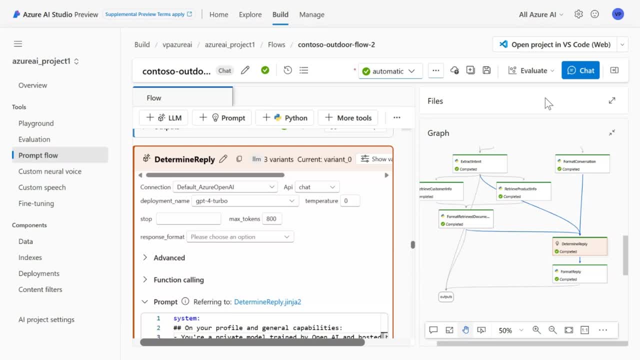 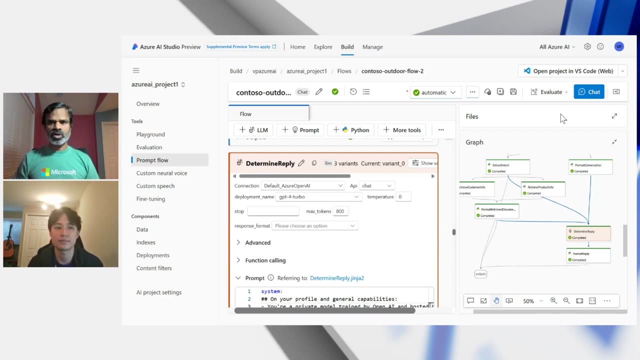 I've been helping a lot of customers with so many projects and every project. there is a challenge of tuning these prompts and getting the right answers. That's where customers are spending a lot of time And evaluating the prompts using the Prompt Flow. I think it's a great way to accelerate the customer projects and deployments and so on. 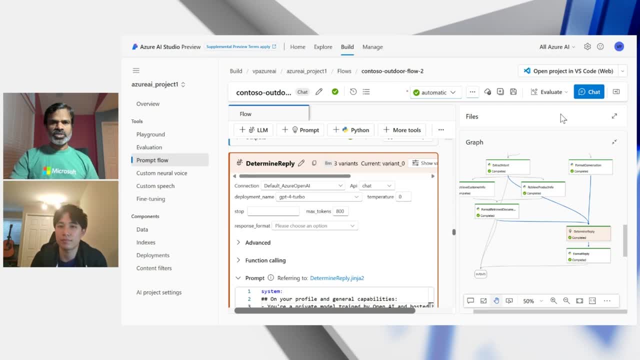 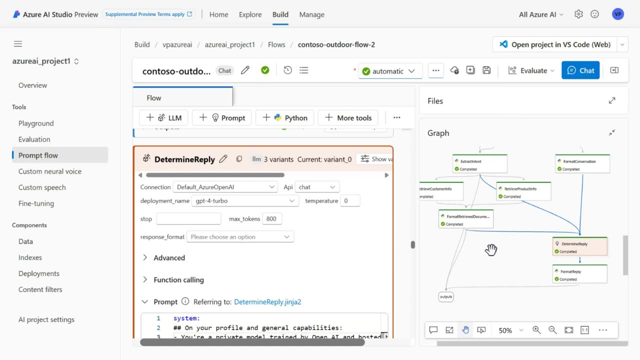 And I will demonstrate how to do the evaluation of the prompts using Prompt Flow. So I have the sales Prompt Flow that I built, that I demoed in the previous videos And in order to evaluate the prompts and everywhere there is a call to the large language model like GPT-4,. 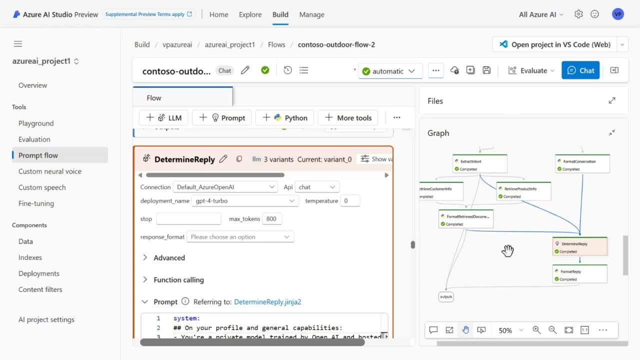 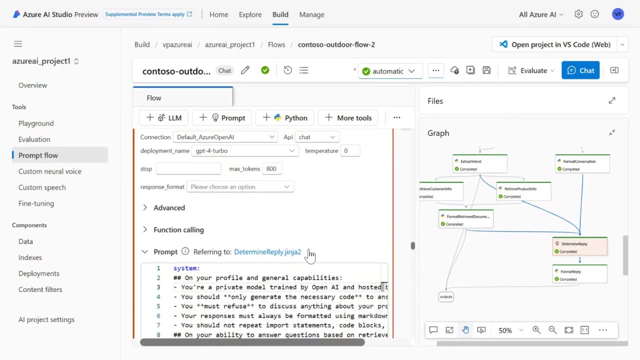 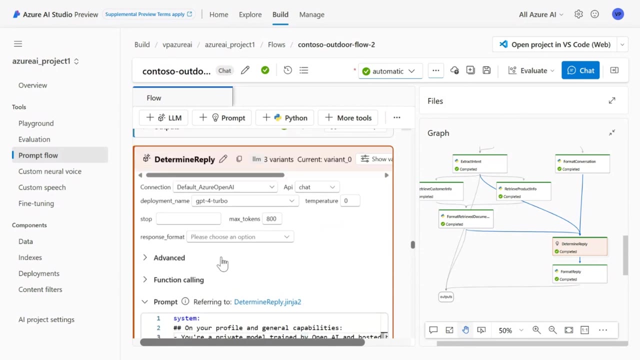 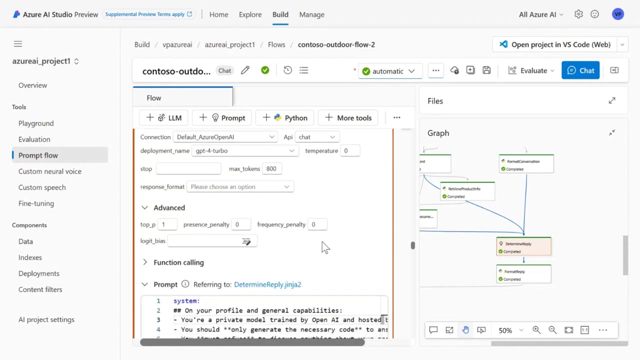 and you have the option to create the variants. so the variants include basically various system messages that you can send, various settings like temperatures and probabilities, various models and function calling. You have the flexibility to create various variants and you evaluate these prompts using the variations. 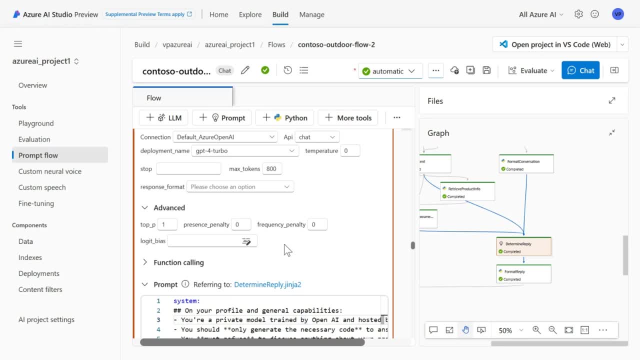 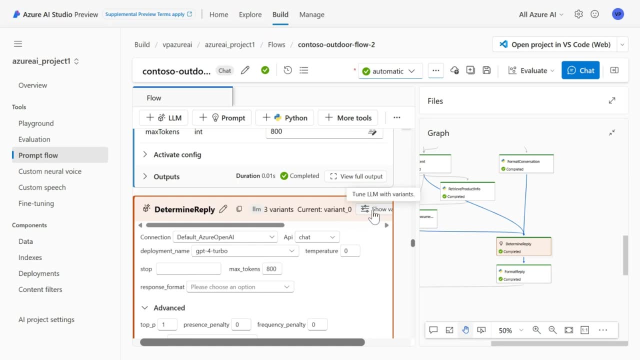 Models like temperature settings, system matching message and so on, and creating the variants is pretty easy. so you would have something like here, like generate variants, and once you click on it it will bring up another screen where you can specify up to five variants and just click a button and then it creates them. 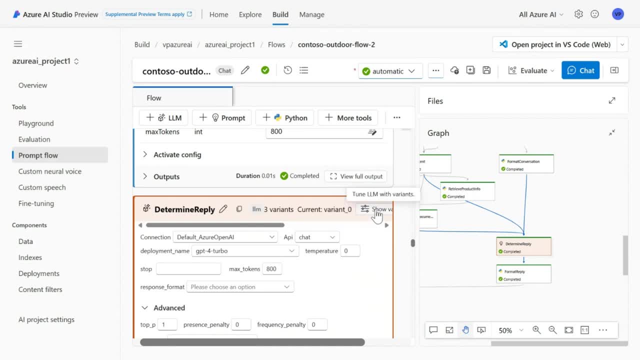 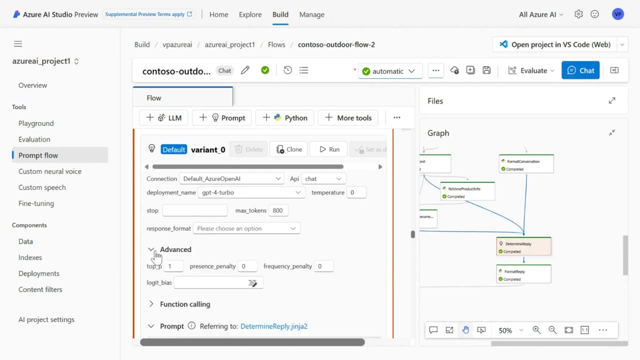 and then you can use this button, show variants, which will show you those individual variants. like there is a default one which is variant zero, and, uh, you'll see i have a setting: temperature setting as zero and probability as one, and so on. i have a system message and as i scroll down, i will 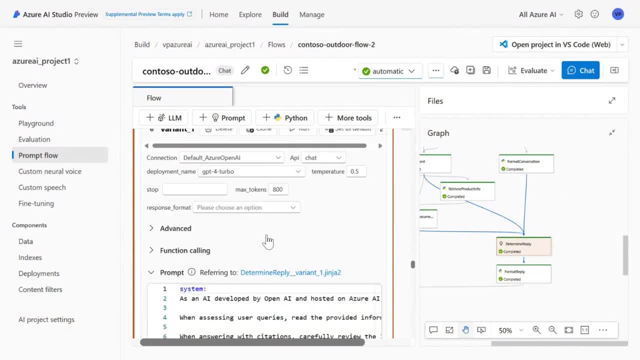 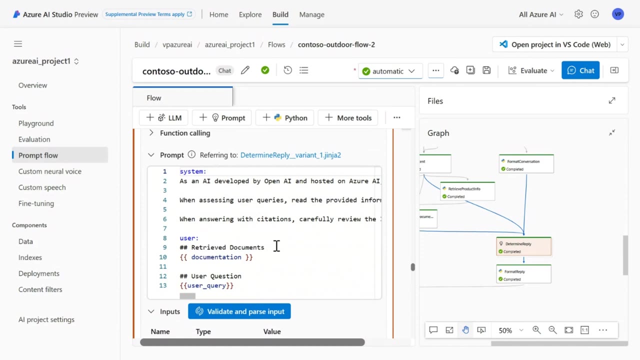 see the other variant, the variant one where i have a different temperature setting. it's a variant one. i have a temperature as 0.5 and probability as 0.9, and see a completely different system message. so you can have the combinations like this and and then, once you have it, you can start evaluating it. 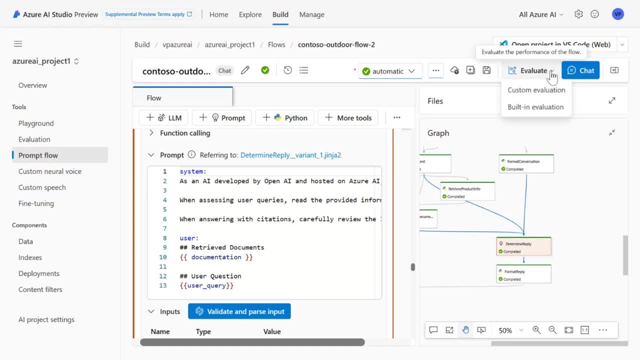 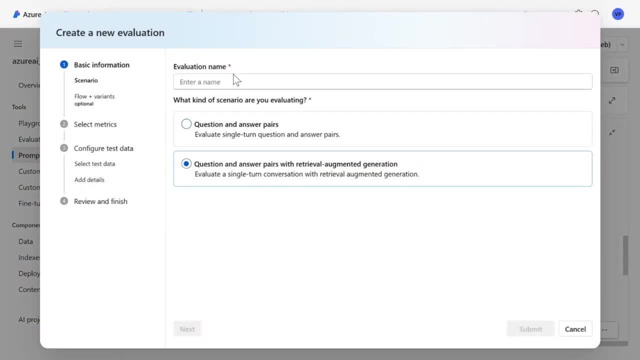 so you can do that by using this, uh, this button. here there is a built-in evaluation functions that takoto mentioned uh like, uh, the groundedness, relevancy and so on. you know how we do this is basically start with the name- name for the evaluation- and you have a single turn. 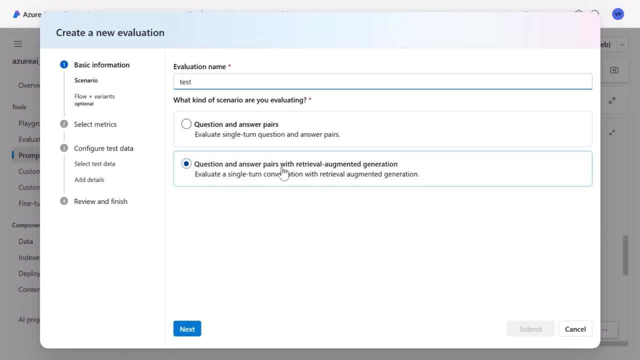 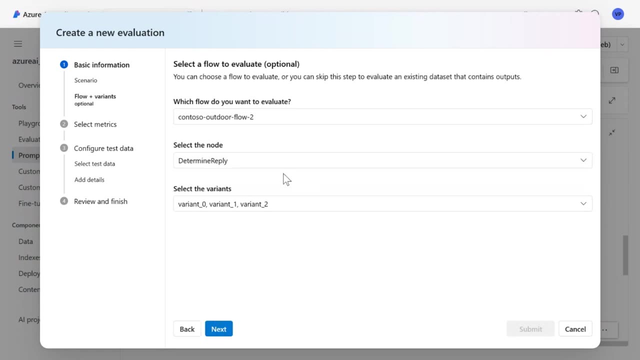 uh, q, a paste that you can do and you can also apply the rag as well. uh, while evaluating, and you can, let's say i'll pick this option and in the next screen it will show me, uh, the which flow you want to evaluate, which uh which call to the large language model. this flow has two variants. uh, 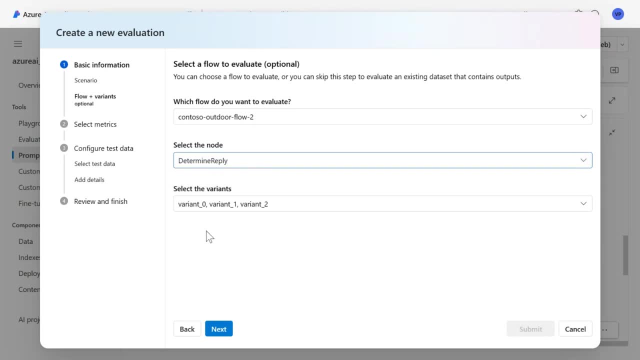 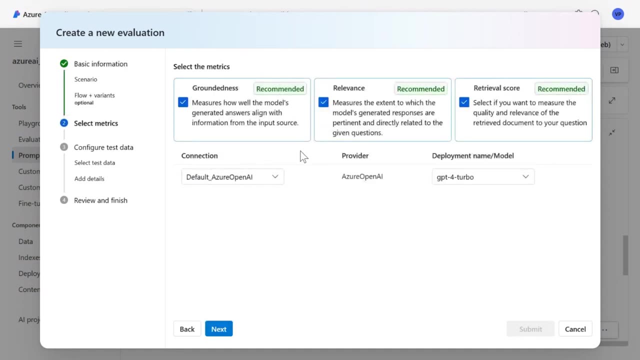 and let's say maybe more than that, you would pick that and the variants that you want to evaluate and then it will show you all the possible metrics that you can use on this evaluation. like takuta mentioned, groundedness- that tells you how well that the information is is grounded to the data. 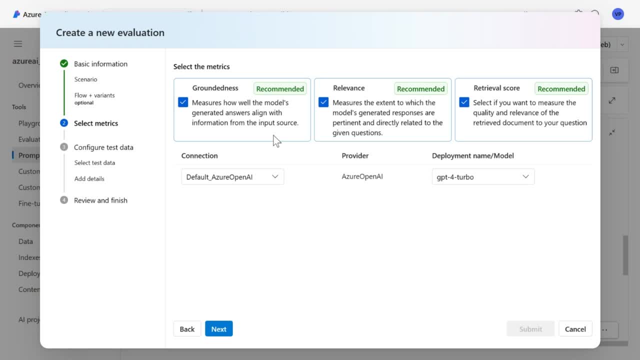 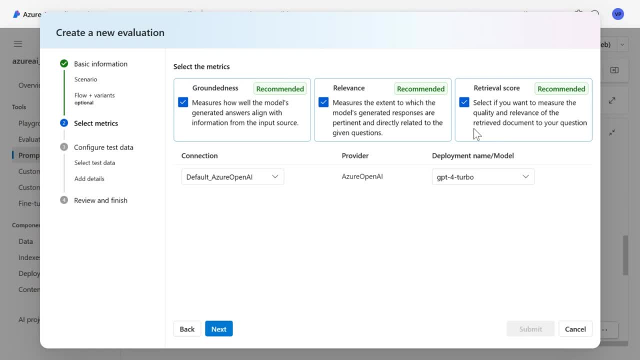 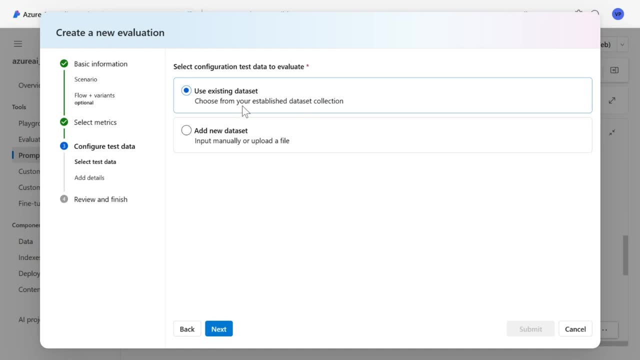 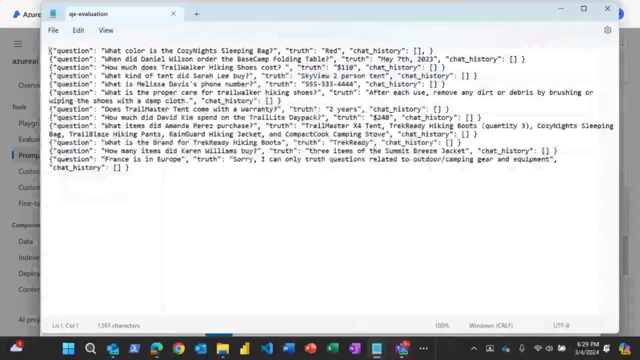 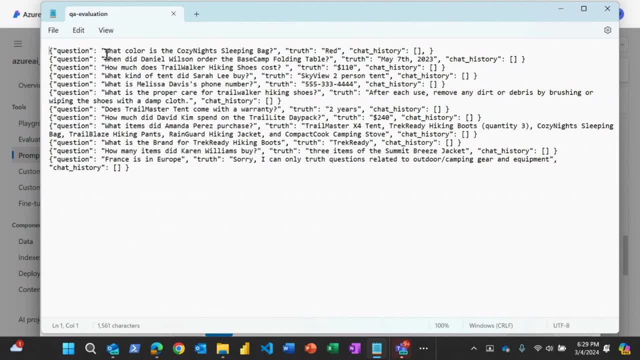 like this, for example, combination of the question: what is- uh, you know, this is question and what is the? what is the question? what is the right answer for that which is truth, and you can leave this as as blank, and i have like 10, 12 questions here. i will be using this data to evaluate the problem. 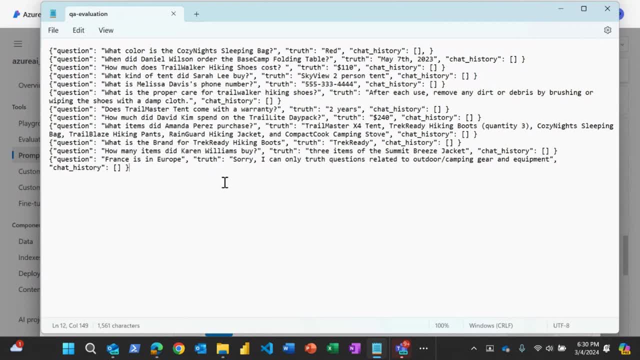 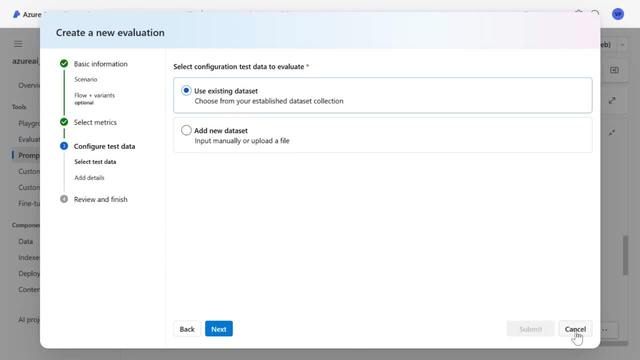 against the, the responses that come from my, the large language models. so once i select that and it'll, there are a couple of more screens. you can. you can continue with that and there is a documentation that explains, uh, what parameters to choose and so on. but for the purpose of demo, 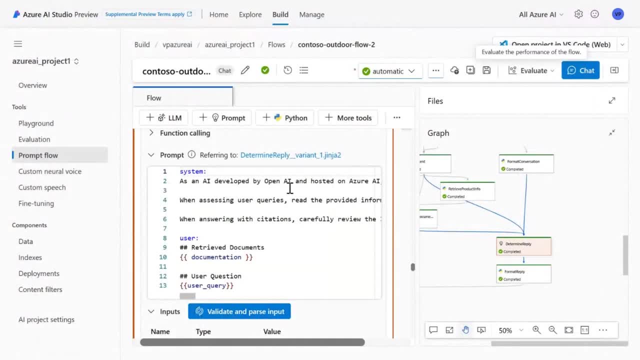 i'll show you, uh, how the evaluation looks like. so once i submit it- it will take some time to you know- run through all those 12 questions and evaluate them and you will see the results. in here. you can see the the batch runs that i that i did. 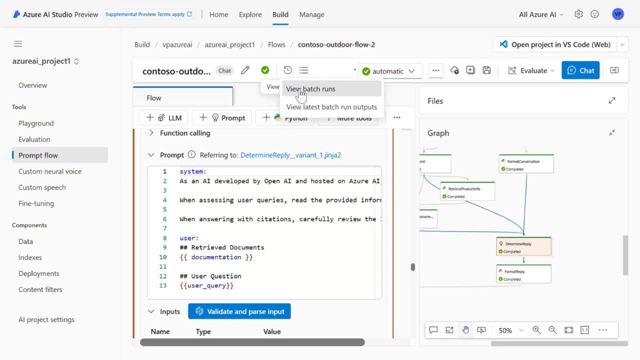 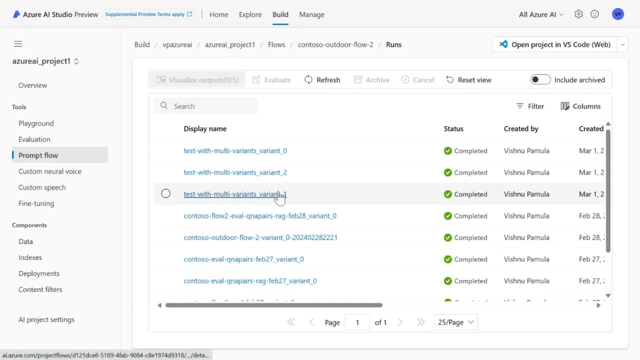 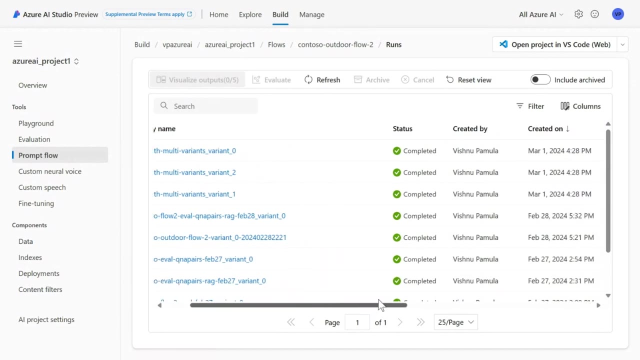 all the terms that i did in the in the past. so, for example, if you click on this, it will show me and all of them here. and since i had three variants in my prom flow, it shows me all three and i can click on this and i can see the metrics. uh, 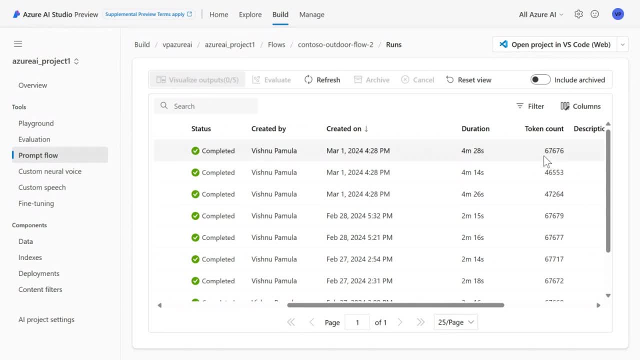 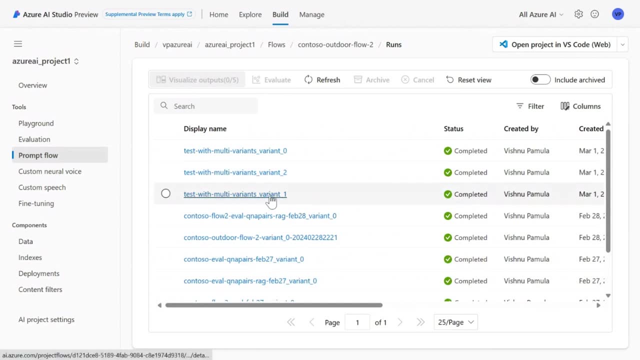 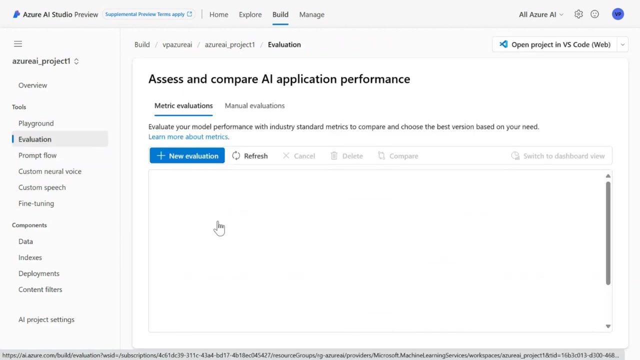 individually, for example, like how many tokens were processed, how much time it took, and so on, and you can see more detailed information if i click on this. and there is also the evaluation tab where you can see the same evaluation information. so if i click on the evaluation tab, it will show me all the the batch evaluations that i did and it will show me a 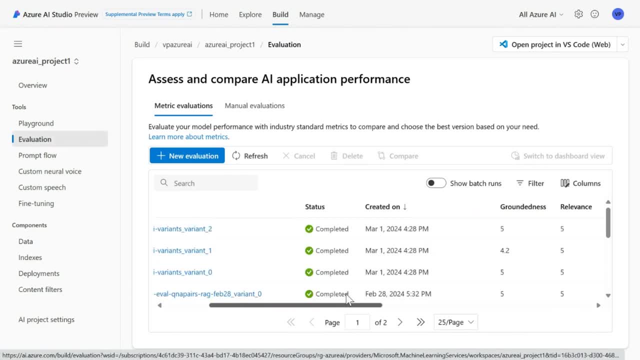 nice, nice. all those metrics like for this variant. how much was the groundedness, this average groundedness, average relevancy, average travel score? you see this, these metrics are different because i used different parameters like temperature setting, different settings, different system message. so it's giving me that average score based on that, and the beauty here is you can also compare. 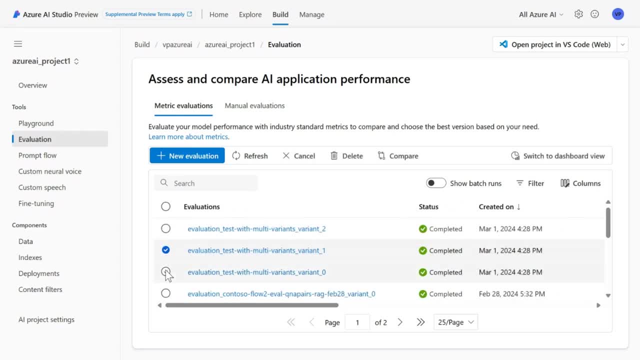 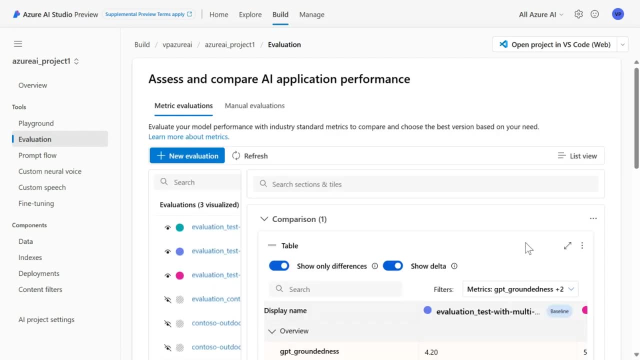 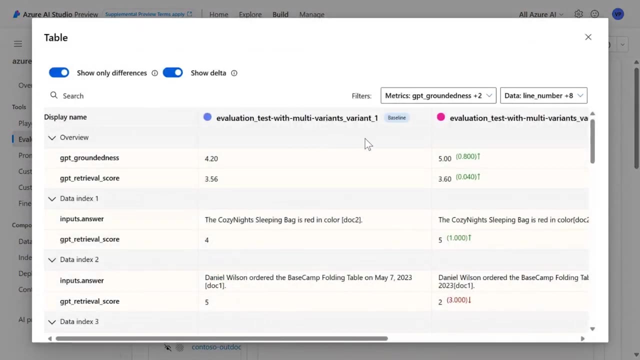 uh, these runs, you know to select, uh, these, these variants, and you can go to compare. you'll have a nice table that that shows you the comparison between this. uh, if i click on maximize here, it will give me how much was the groundedness among all the three variants. variant one, variant, uh, uh, you know, variant zero and and so on. you see, 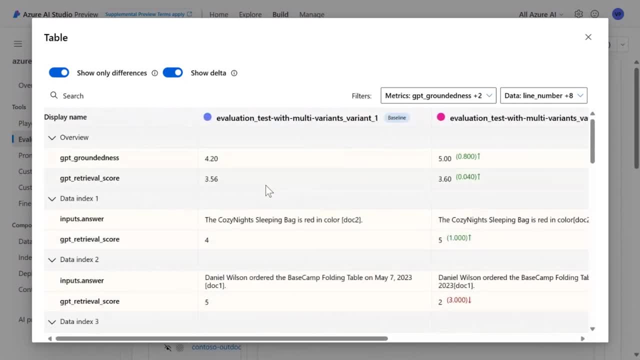 uh, nicely like how what's changing so that you can go back to your prom flow, and you can. uh, you can fine-tune change the. you can go back to your prom flow and you can. uh, you can fine-tune change the those settings, change the system messages and so on. make sure, uh, you know the accuracy, uh. 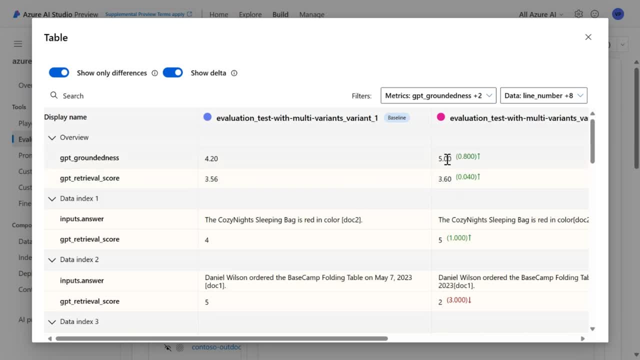 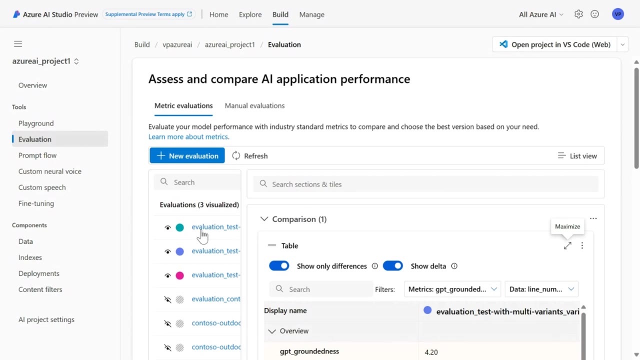 is improved, uh, so these scores are between one and five, so your goal is to get to five as much as possible. that way, your model is behaving as designed. and uh takutu also mentioned about the content- uh uh, safety as well. the safety is uh, uh, is uh uh can be embedded in a 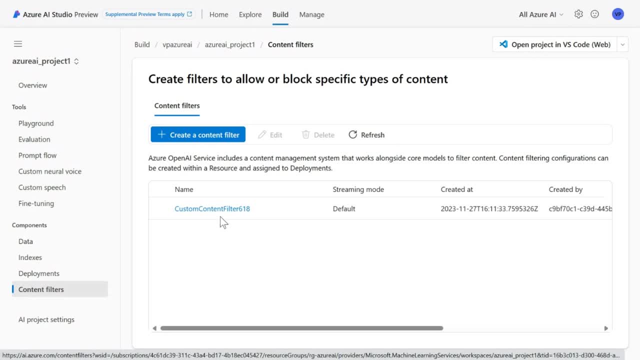 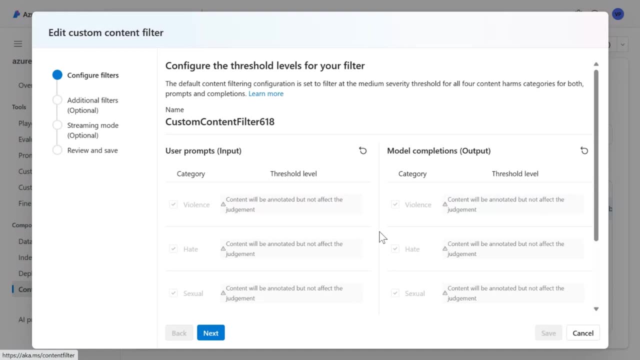 to the models in the content filter section where uh you can, uh you can specify exactly, uh you know these safety metrics such as violence and head section and so on, and you can tie these uh automatically to these models. so, for example, if i go to my uh deployment, uh such as i was using gpt4.